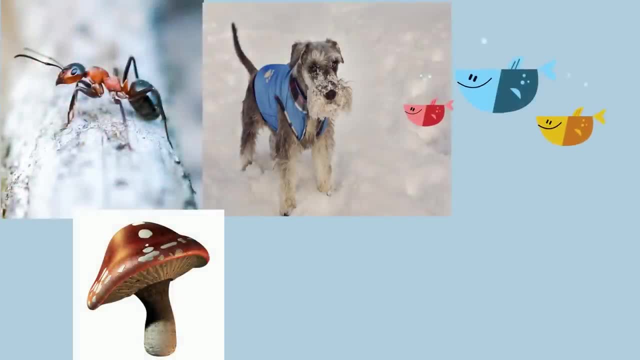 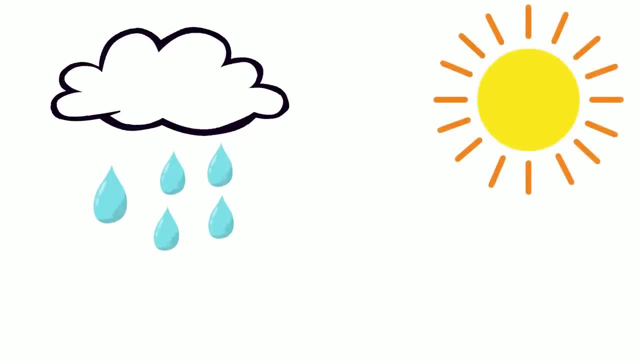 Ants, dogs, fish, mushrooms, plants and this praying mantis are examples of biotic factors. Clouds, sunshine, water and diamonds would be examples of abiotic factors. Let's apply the idea of biotic and abiotic factors to another organism, one that a field ecologist might be likely to study. 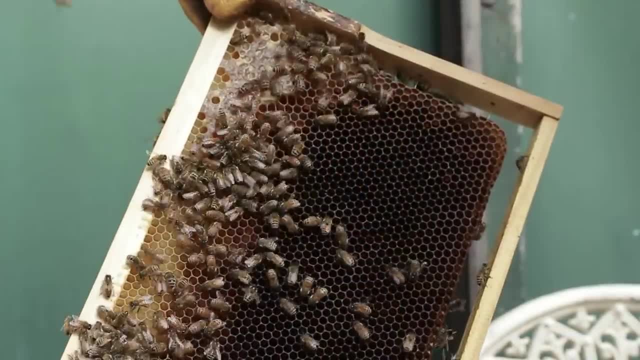 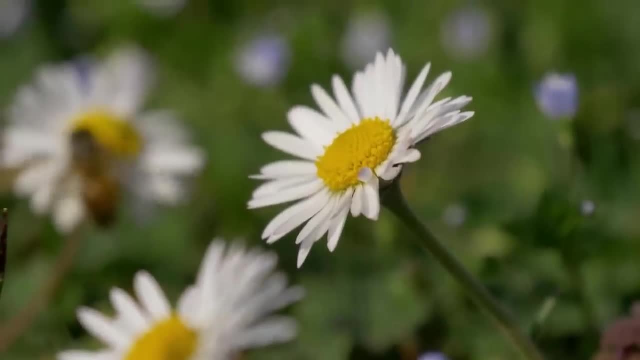 For years, the population of honeybees has been declining in North America. Bees are very important to their environment because they help pollinate plants. Understanding the main factors responsible for this decline in bees help ecologists form plans to protect the species. 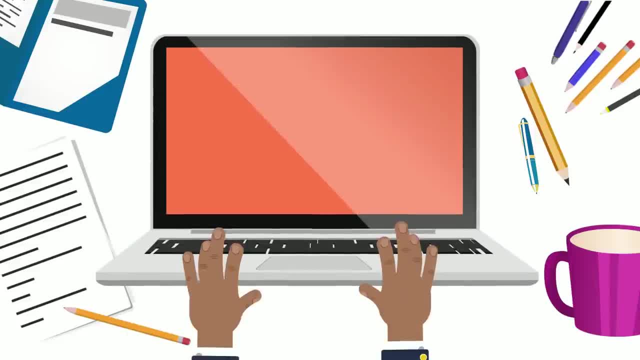 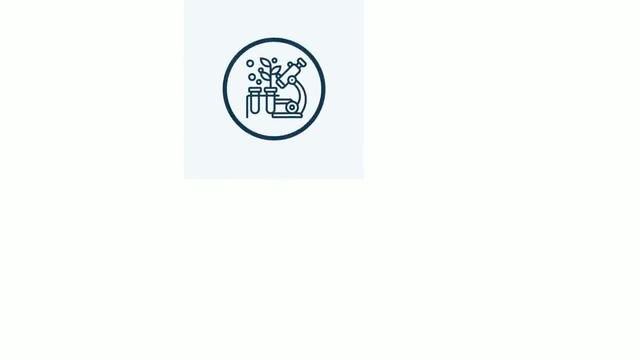 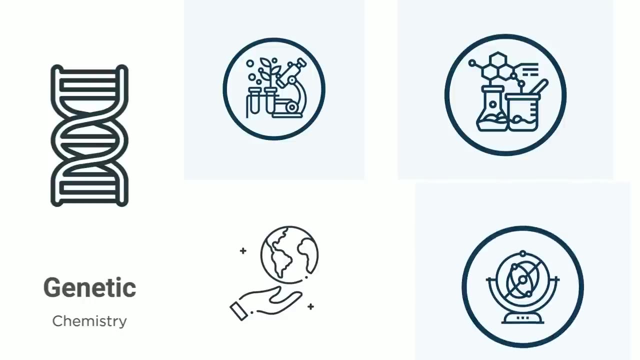 Ecologists may ask a question like this: Why is the bee population declining? Ecologists would then draw on many areas, including biology, genetics, earth science, chemistry and physics, to name just a few, to help solve this question. Ecology can be studied at five broad levels. 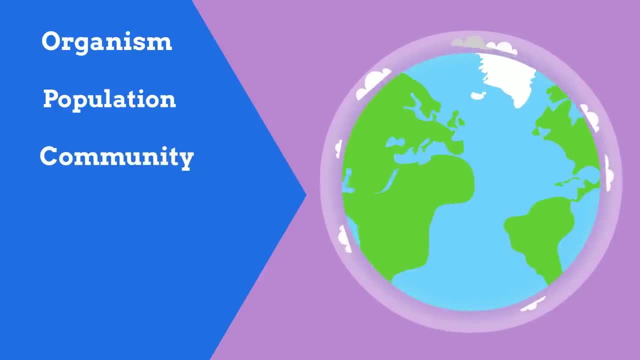 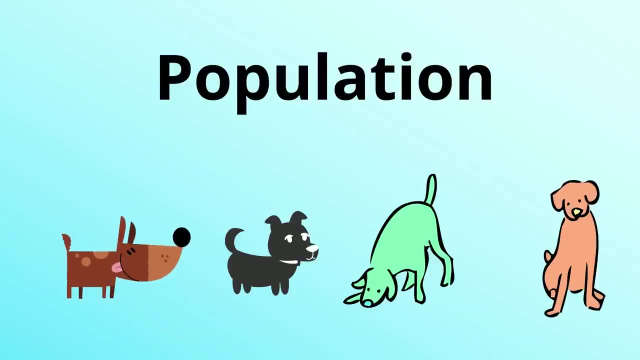 The organism, population, community, ecosystem and biosphere. Let's take a look at each level. Organism- An organism can range from a single protist to a large animal like an elephant. Population is a group of organisms of the same species that live in the same area at the same time. 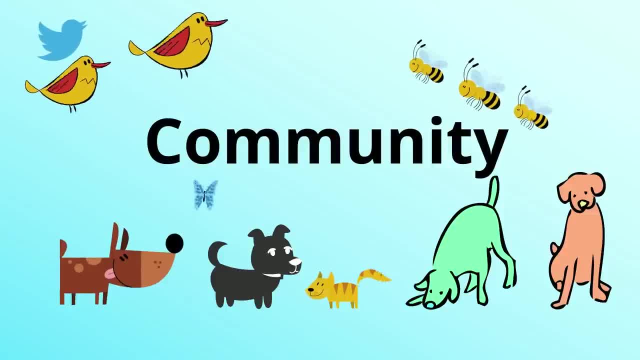 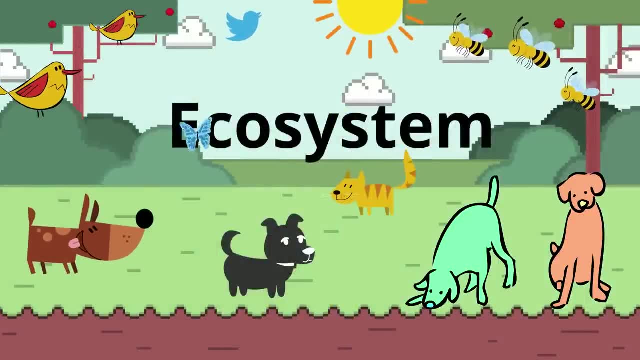 A community, a biological community consists of all the populations of different species that live in a given area. An ecosystem consists of all the organisms in an area, the community and the abiotic factors that influence the community And biosphere. This is planet earth viewed as an ecological system. 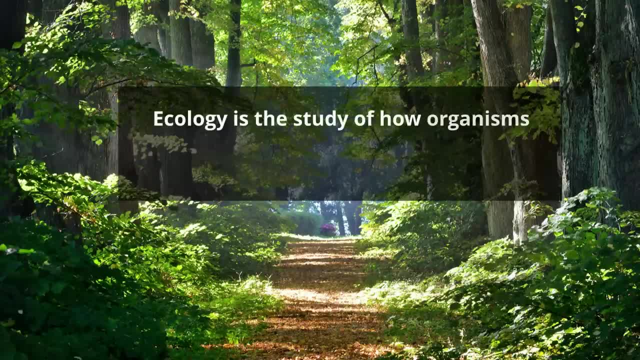 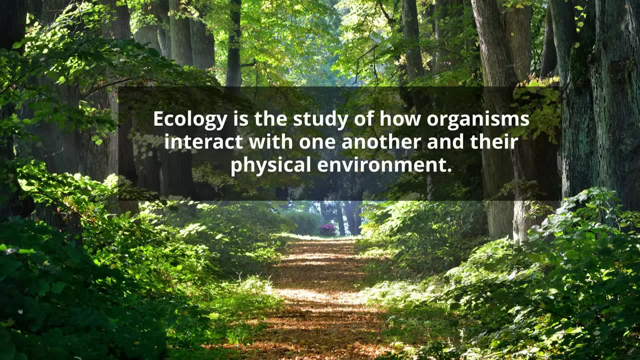 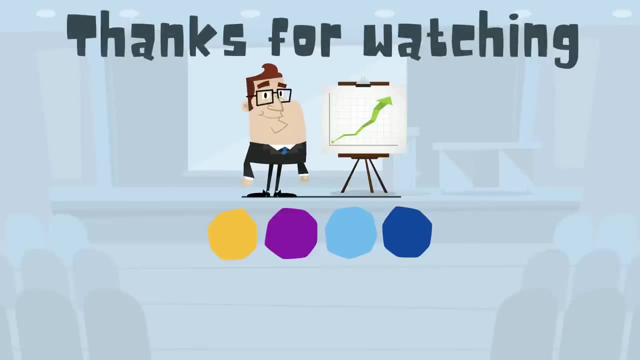 So, in summary, ecology is the study of how organisms interact with one another and their physical environment. And remember: kindness always multiplies kindness. Thanks for watching, and MooMooMath uploads a new math and science video every day. Please subscribe and share.